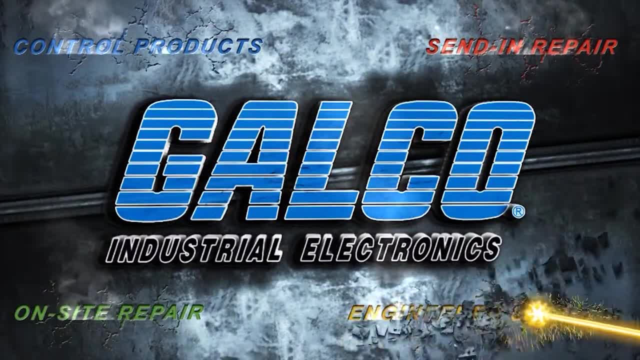 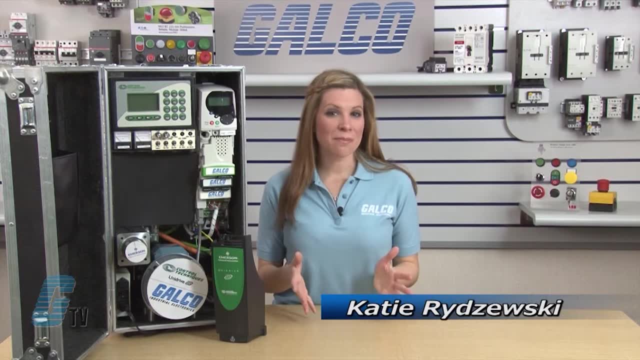 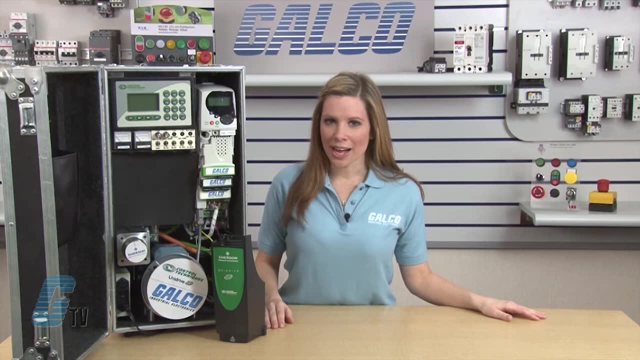 Welcome to G-TV. Today I'll be showing you Emerson Control Techniques- SM Feedback Option Modules. The Feedback Option SM Modules can be used with motor drives such as Mentor MP, Quantum MP, Unidrive SP and Digitex ST. The SM Feedback Option Modules supplement the standard interfaces. 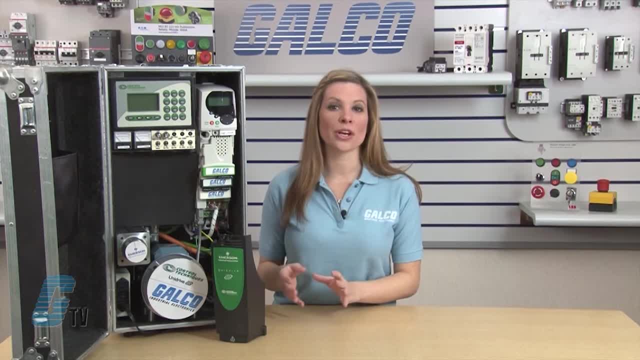 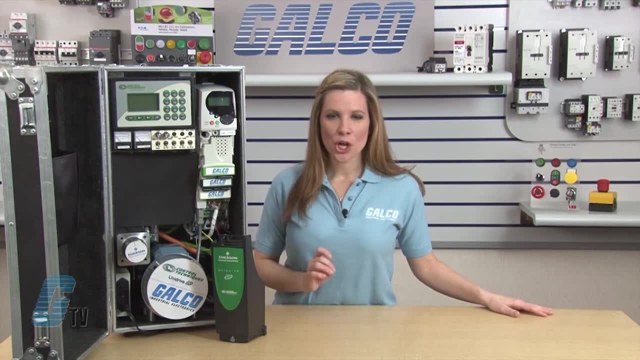 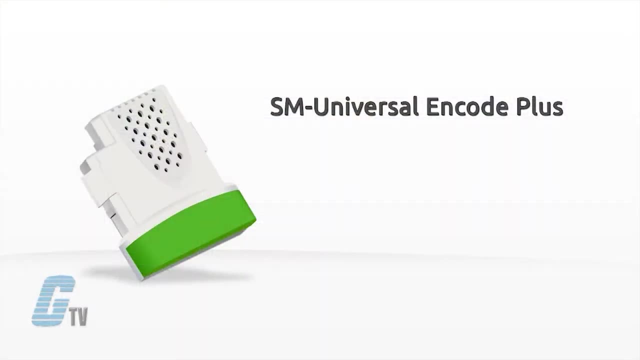 on Control Techniques drives enhancing their control and automation capabilities. The modules enable connection to multiple measurement sources simultaneously utilizing a wide range of position and speed measurement device types. The light green SM Universal Encode Plus provides the drive with an additional speed measurement device type. The light green- SM Universal Encode Plus provides the drive with an additional speed measurement type. The light green- SM Universal Encode Plus provides the drive with an additional speed measurement device type. The light red- SM Universal Encode Plus provides the drive with an additional speed measurement device type. The light green- SM Universal Encode Plus provides. 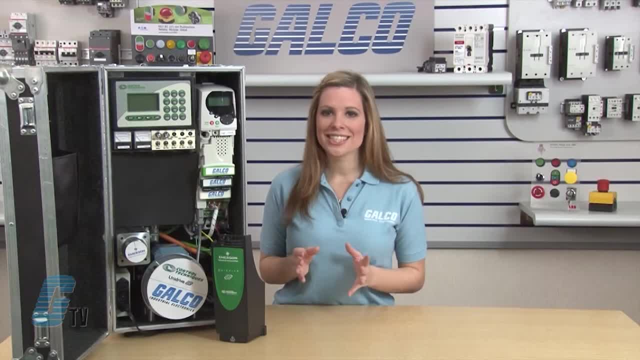 the drive with an additional key set of an additional feedback port with the same functionality as the base drive, supporting SYN costs with commutation, quadrature-incremental pulse & direction and SSI. The module also provides a simulated encoder output that can be programmed. 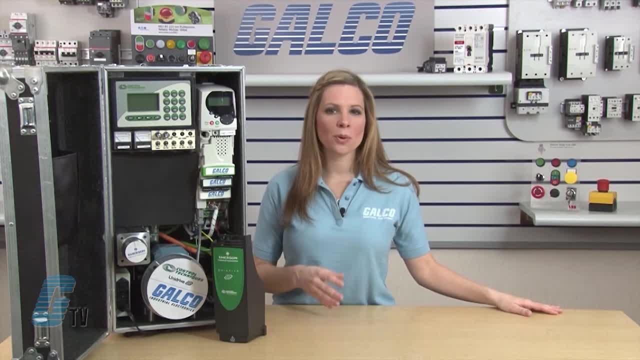 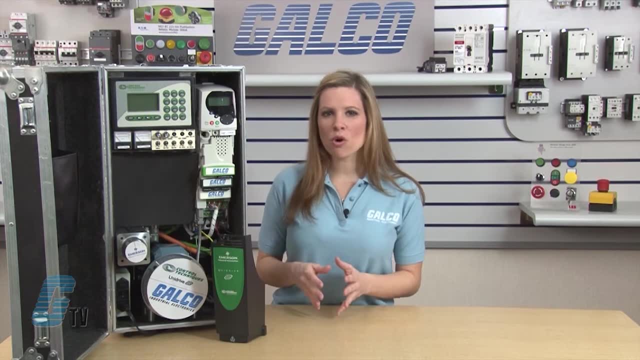 to operate in quadrature-incremental pulse & direction combos and another ECM together. Endless stratification either is available via the differential selector switch and can be applied at any time using the す. The Brown SM Encoder Plus is an interoperable proposal framework with the following doubling 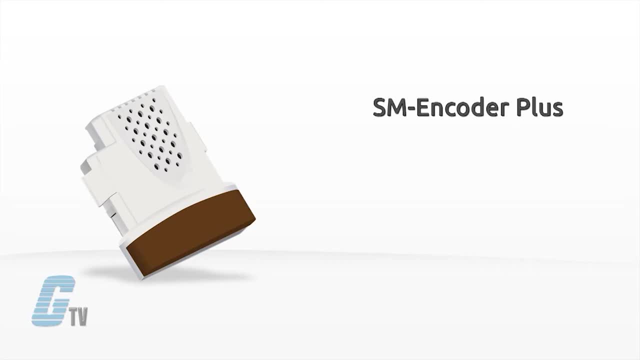 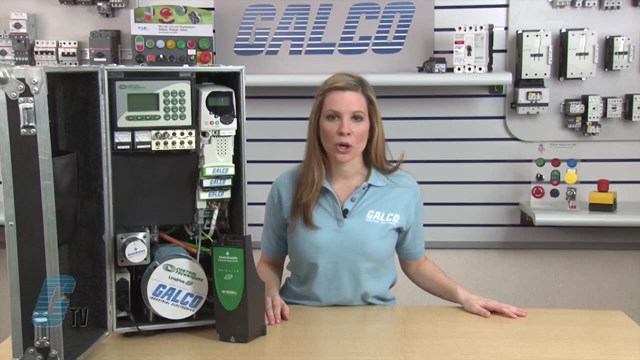 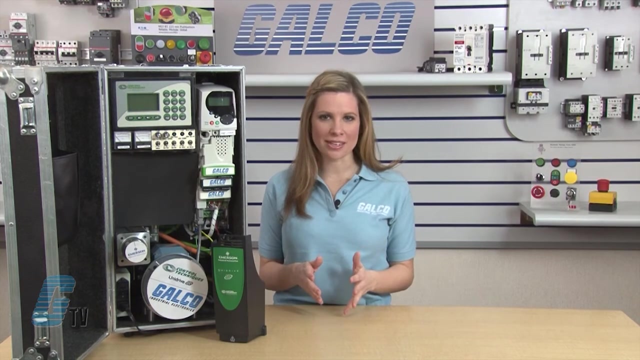 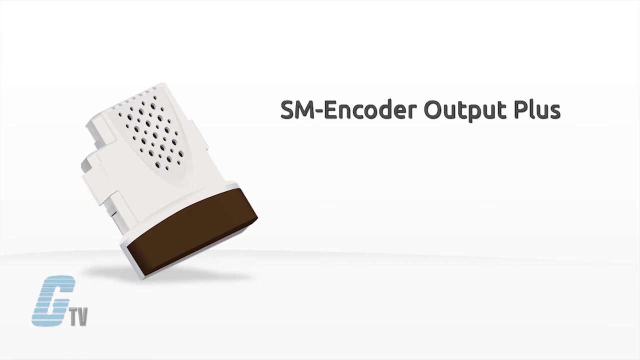 filters, An incremental encoder input option module. it supports encoder inputs such as closed loop vector, motor feedback, quadrature encoder input and marker pulse. It also supports incremental encoders with frequency and direction signals and incremental encoders with forward and reverse signals. The darker brown module is the SM encoder output plus. 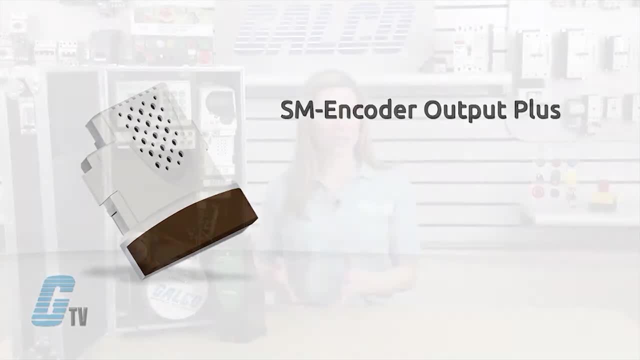 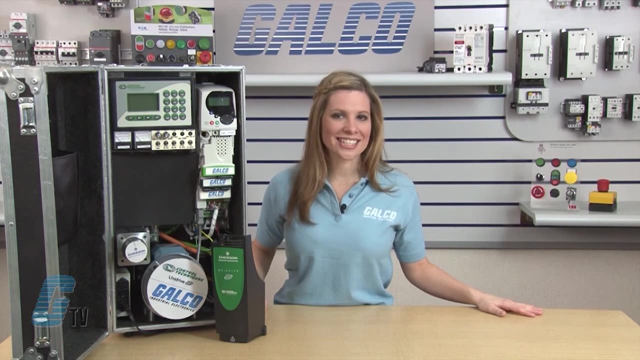 It is an incremental encoder input and output option module to enable connection with external motion controllers. It supports the same encode inputs as the SM encoder plus. The simulated encoder output types for this module are quadrature, frequency and direction- forward and reverse, and marker lock.